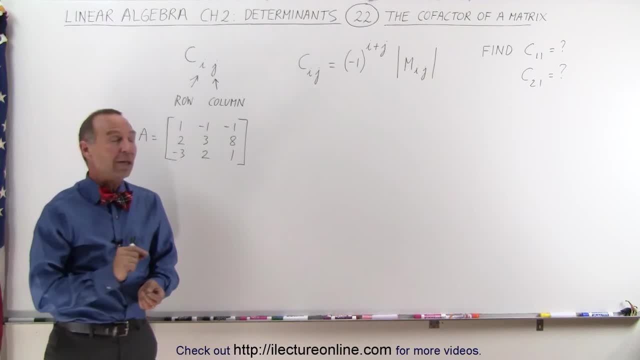 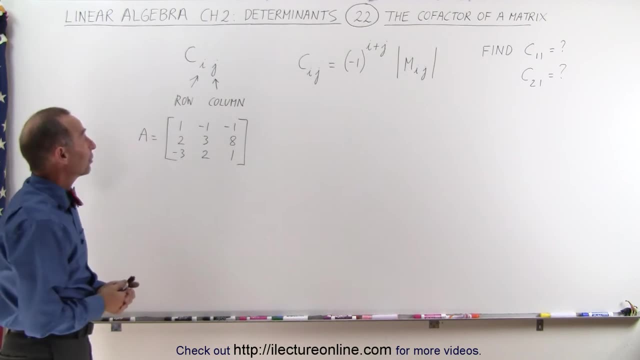 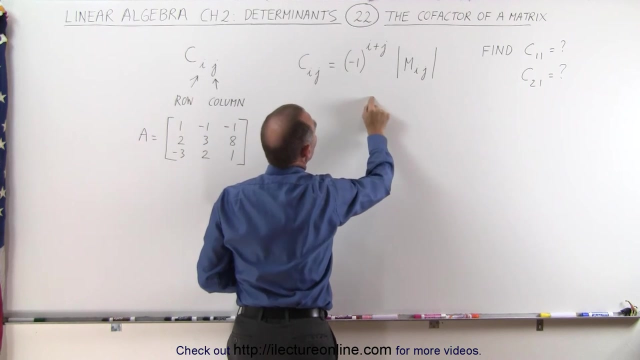 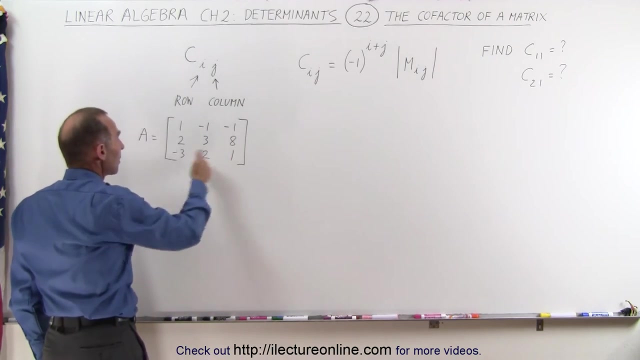 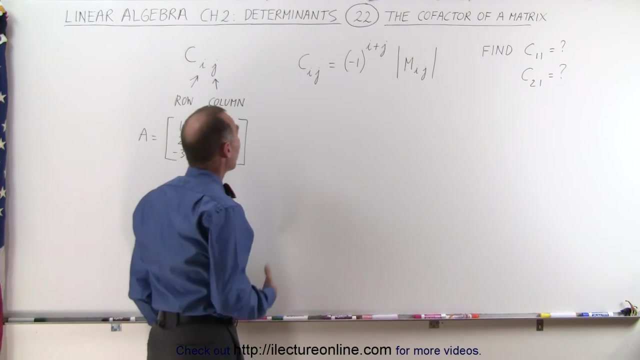 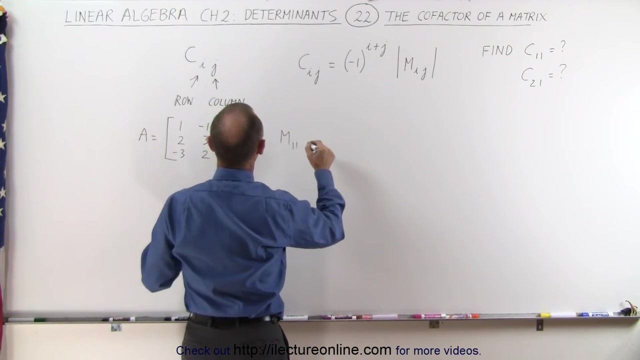 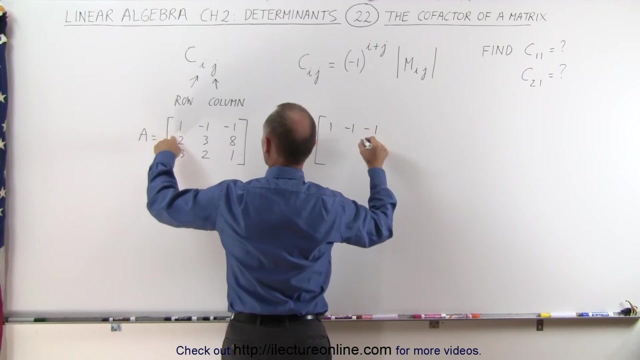 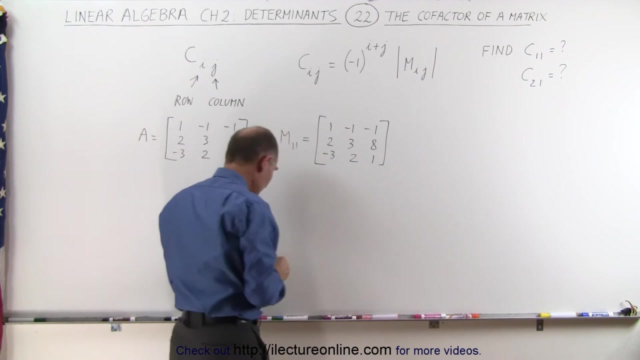 Welcome to ElectronLine. Now that we know how to find the minor of a matrix, we're going to find the cofactor of a matrix. And here's the definition of a cofactor. Well, first of all, we write it with a c and the subscripts i and j. i is the row, j is the column. And the definition is that cij is equal to negative 1 raised to the i plus j power times the determinant of the minor ij. Here we have the matrix A, which is the 3 by 3 matrix, and we're going to find c11 and c21. Well, first of all, what we need to find is we need to find m11. m11 can be found by taking the original matrix here, the A matrix. Let's write down all the elements. 1, minus 1, minus 1. 2, 3, 8. Minus 3, 2 and 1. And let's get rid of the first row and the first column. 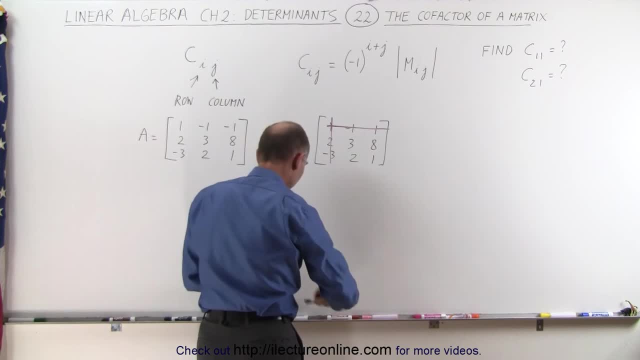 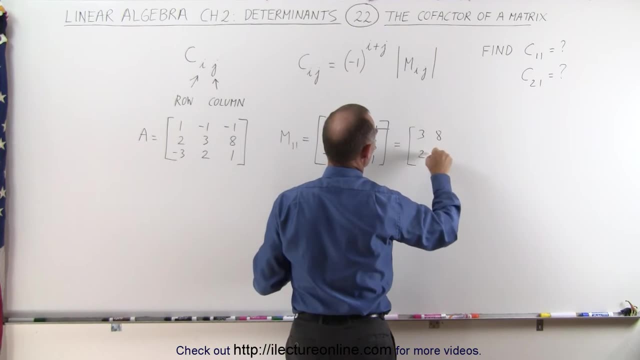 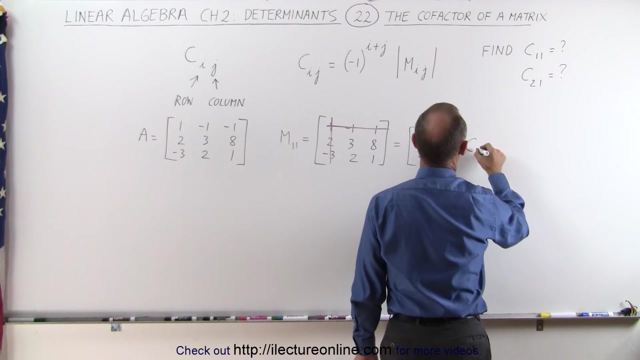 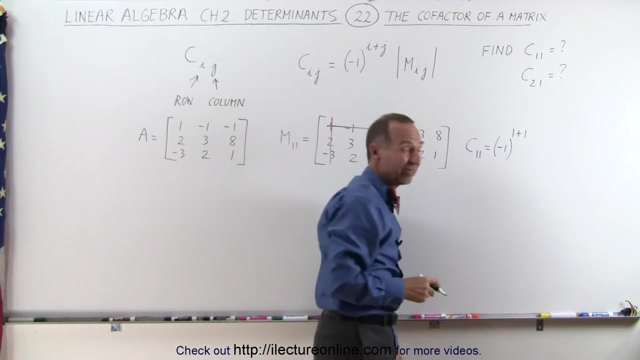 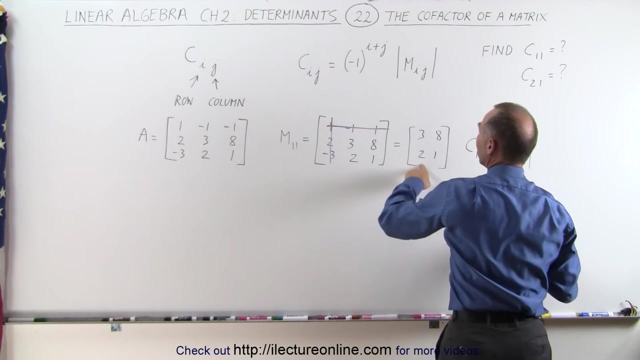 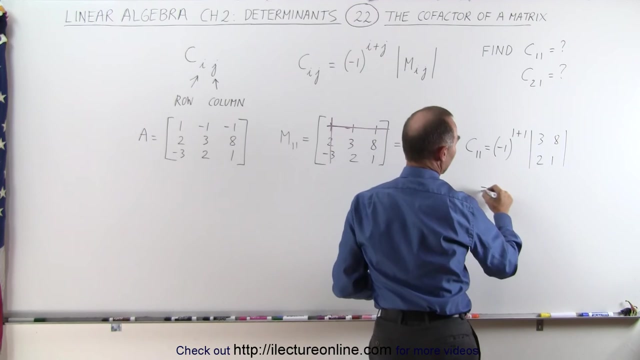 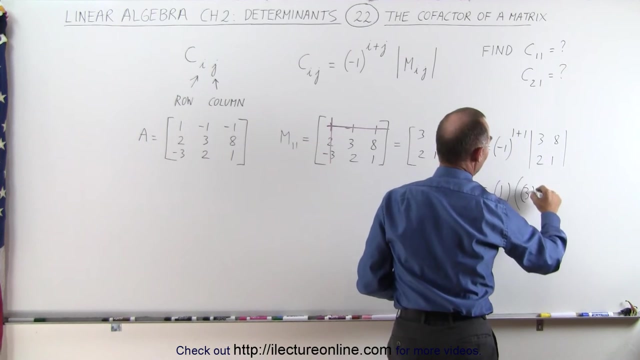 Here's the first row, there's the first column, which means that we end up with this matrix right here. This is equal to the matrix 3, 8, 2 and 1. And now we're ready to find c11, the cofactor of that matrix. And so c11 is going to be equal to minus 1 raised to the 1 plus 1 power. So that's raised to an even power, that becomes a positive 1, times the determinant of this minor, which is 3, 8, 2 and 1. This therefore becomes equal to a positive 1 times, and here you're going to multiply these diagonals, 3 times 1 minus 8 times 2, which is equal to 3 minus 16. 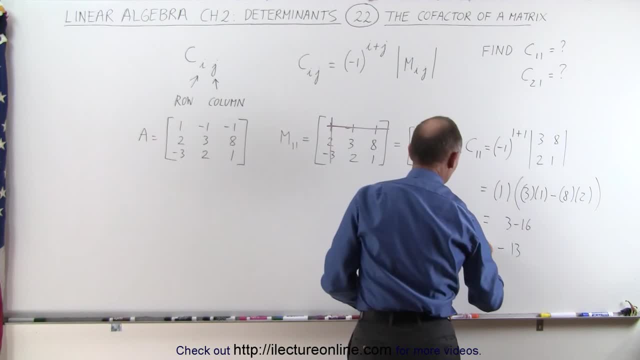 Which is minus 13. Which means that the cofactor c11 equals minus 13. 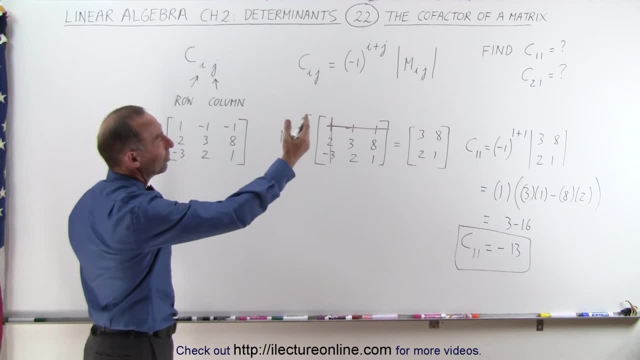 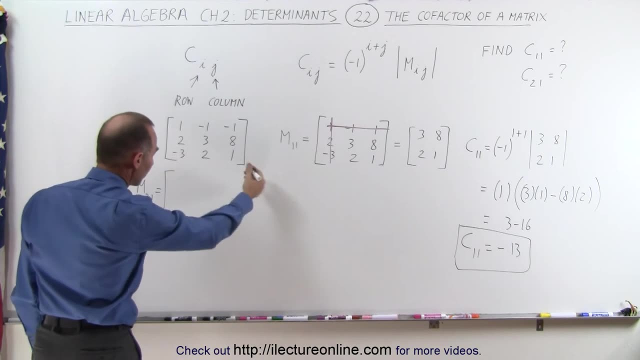 Just so we can get the hang of it, let's do the second one, c21. And therefore we first have to find m21, which is equal to, again, you're going to repeat the same matrix. 1, minus 1, minus 1. 2, 3, 8. Minus 3, 2 and 1. I'd like to use a different color pen. 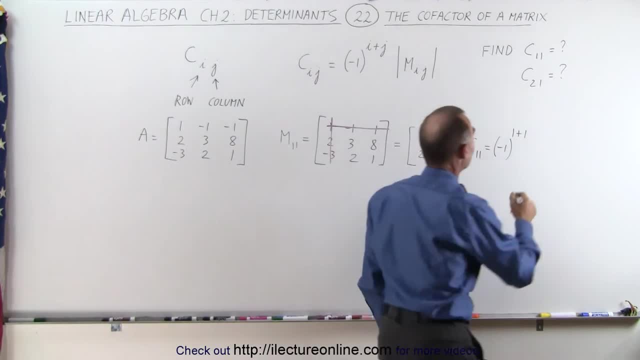 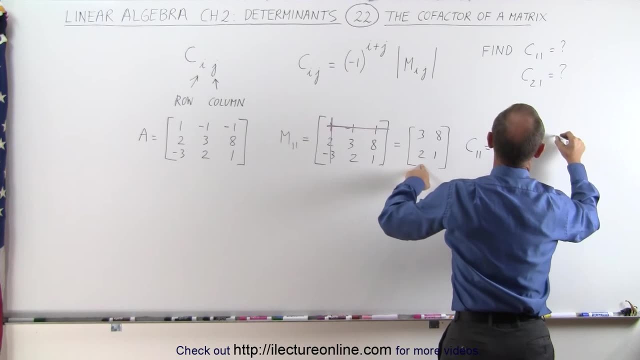 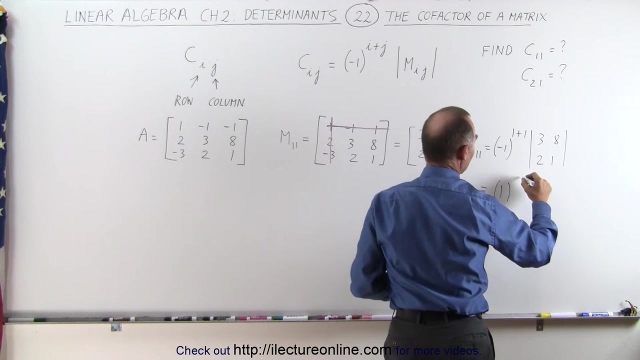 So that's raised to an even power, that becomes a positive 1, times the determinant of this minor, which is 3,, 8,, 2 and 1.. This therefore becomes equal to a positive 1 times. and here you're going to multiply these diagonals. 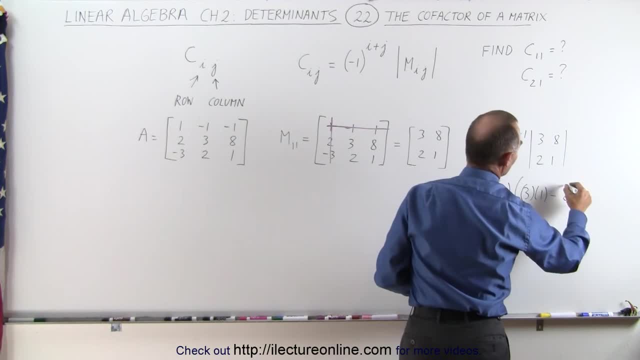 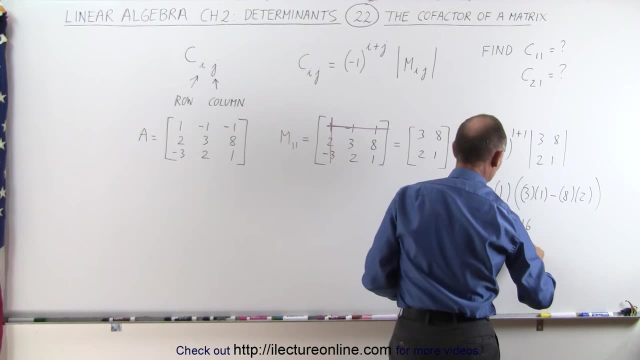 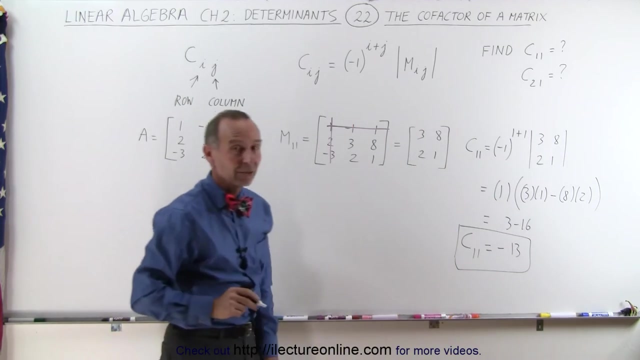 3 times 1 minus 8 times 2,, which is equal to 3 minus 16.. Which is minus 13.. Which means that the cofactor c11 equals minus 13.. Just so we can get the hang of it, let's do the second one, c21.. 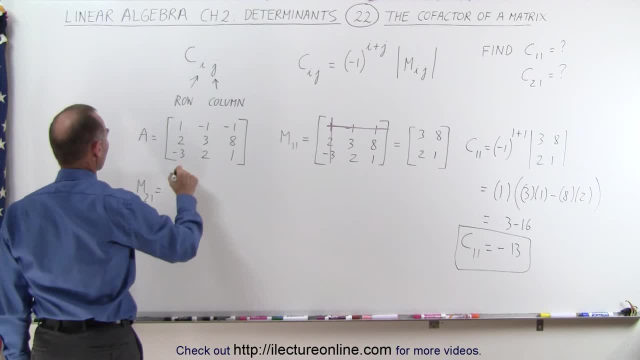 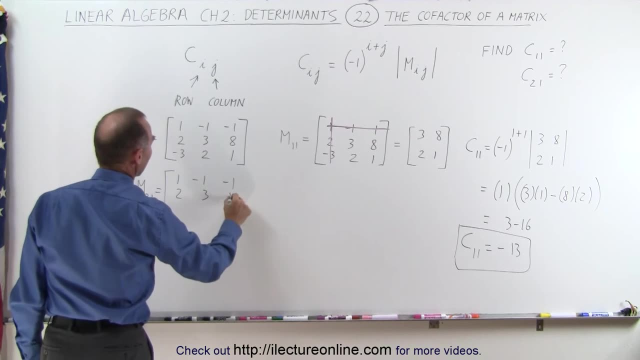 And therefore we first have to find m21, which is equal to. again, you're going to repeat the same matrix: 1, minus 1, minus 1.. 2, 3, 8.. Minus 3, 2 and 1.. 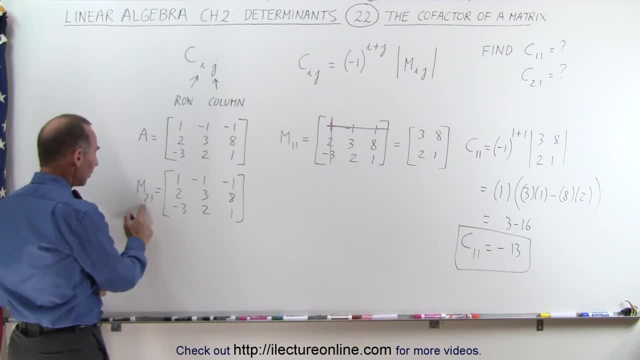 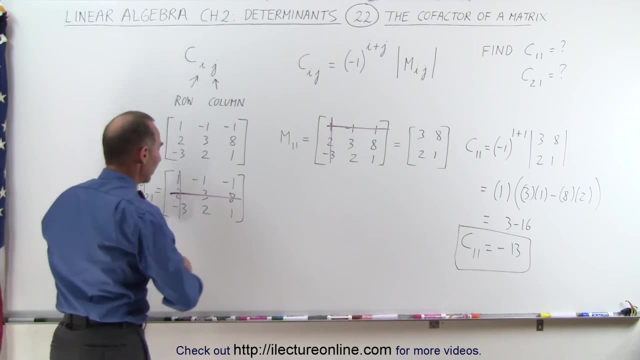 I'd like to use a different color pen. Let's get rid of the second row in the first column. Second row, first column. You're left with these four elements, which means that the minor matrix will now look like this: A minus 1, minus 1,, 2 and 1.. 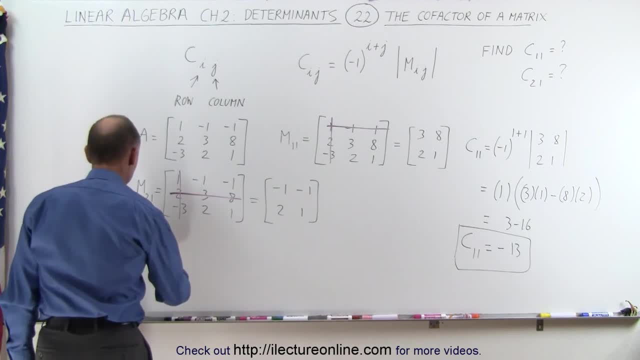 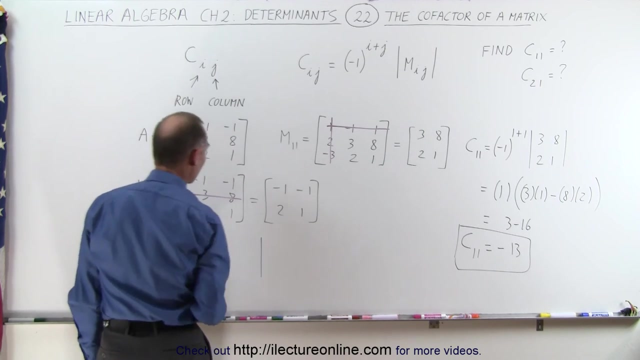 And now what we have to do is the cofactor 2, 1 is equal to minus 1 raised to the 2 plus 1 power, And notice that this is an odd power, so this will become negative Times. the determinant of the minor matrix. 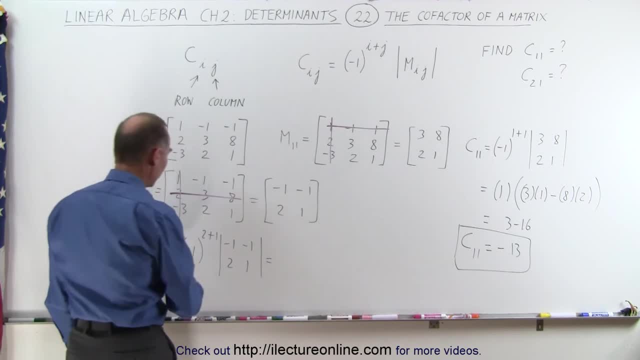 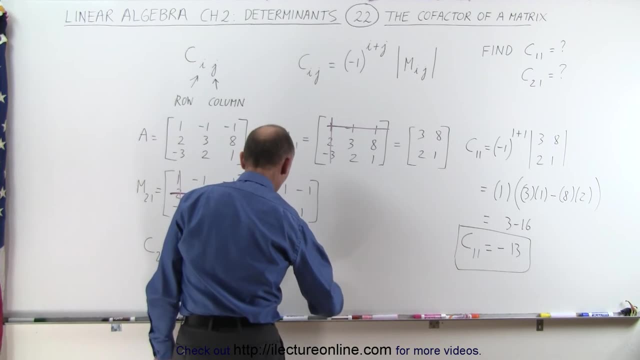 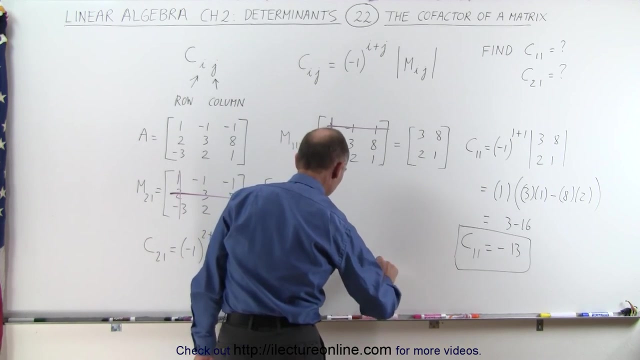 minus 1, minus 1, 2 and 1.. So this becomes a minus 1 times you multiply the cross diagonals. that would be a minus 1 times a 1, minus when you multiply those together: minus 1 times 2.. 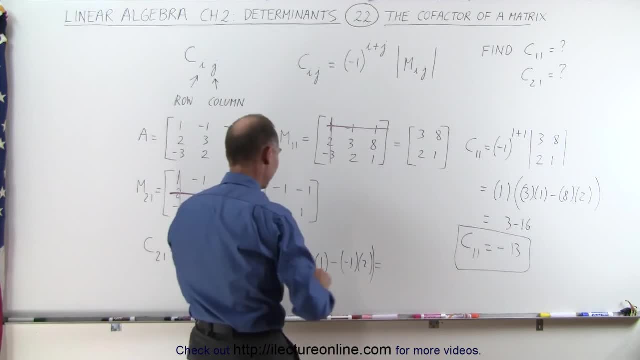 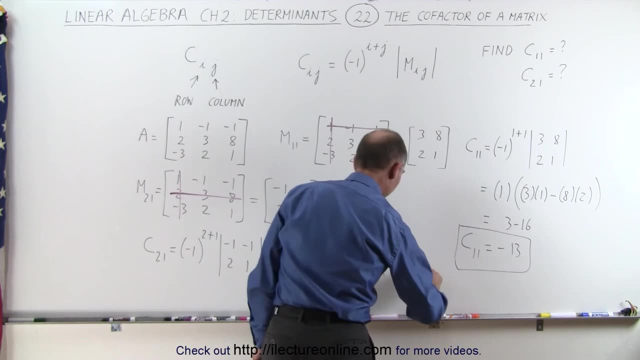 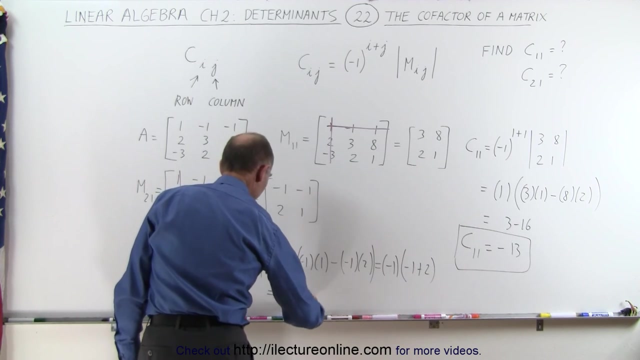 So this becomes a closing parentheses. this becomes a minus 1 times minus 1, and a minus times a minus is plus 2.. So this becomes minus 1 times a plus 1,. this is equal to minus 1 times a plus 1,. 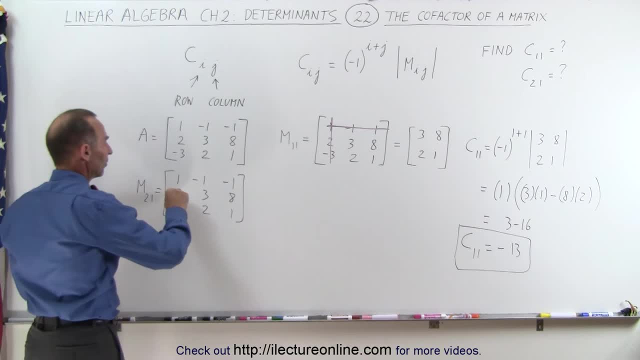 Let's get rid of the second row in the first column. Second row, first column. 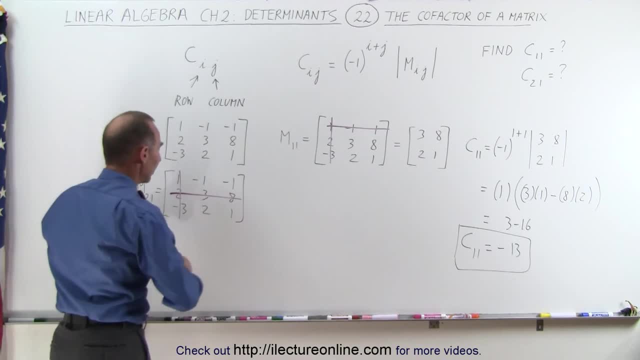 You're left with these four elements, which means that the minor matrix will now look like this. 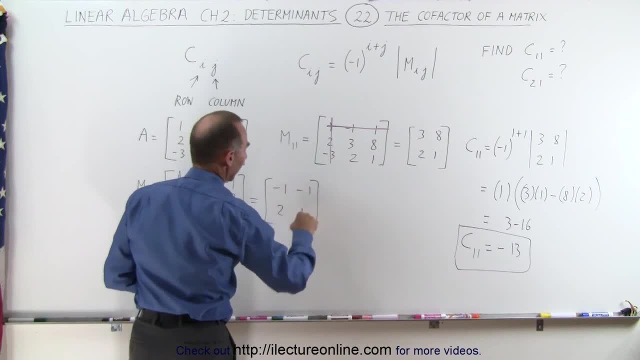 A minus 1, minus 1, 2 and 1. And now what we have to do is 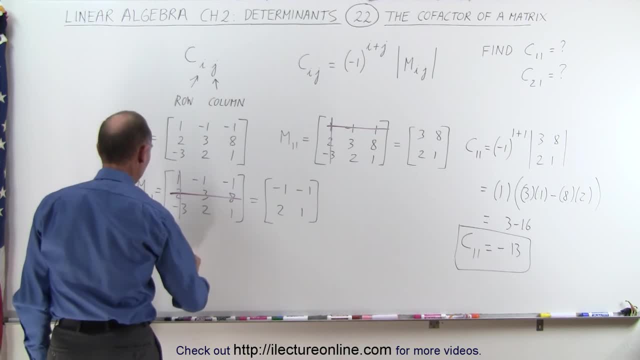 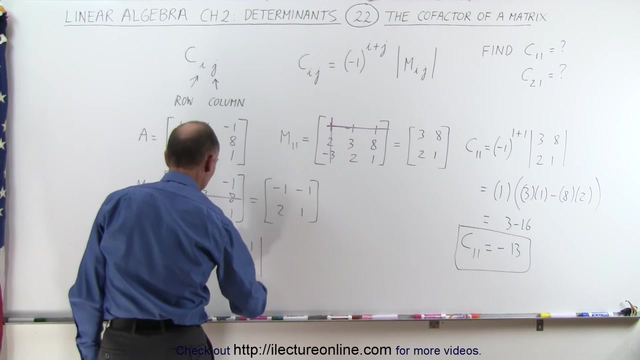 the cofactor 2, 1 is equal to minus 1 raised to the 2 plus 1 power. And notice that this is an odd power, so this will become negative. Times the determinant of the minor matrix, minus 1, minus 1, 2 and 1. 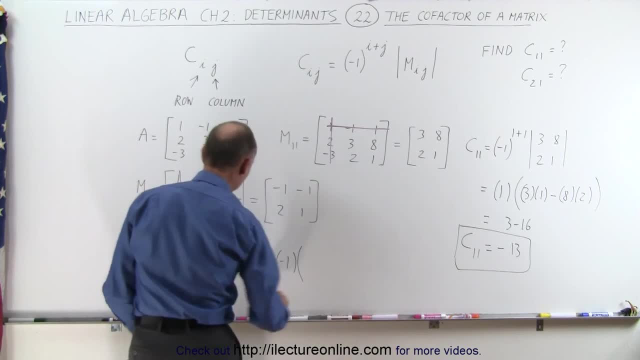 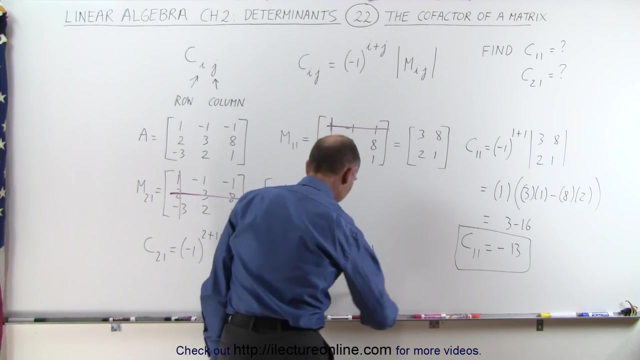 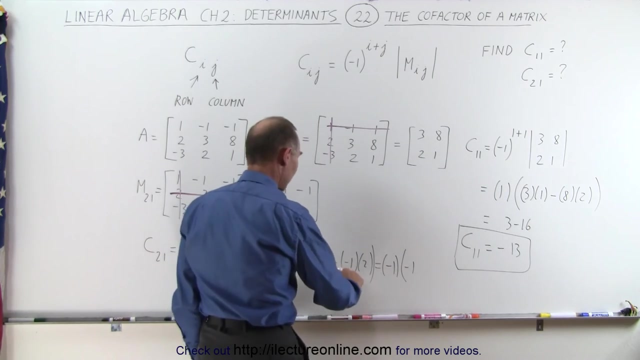 So this becomes a minus 1 times, you multiply the cross diagonals, that would be a minus 1 times a 1, minus, when you multiply those together, minus 1 times 2. So this becomes a, closing parentheses, this becomes a minus 1 times, minus 1, and a minus times a minus is plus 2. 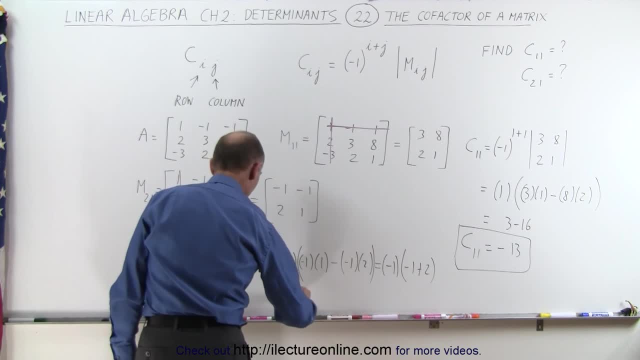 So this becomes minus 1 times a plus 1, this is equal to minus 1 times a plus 1, 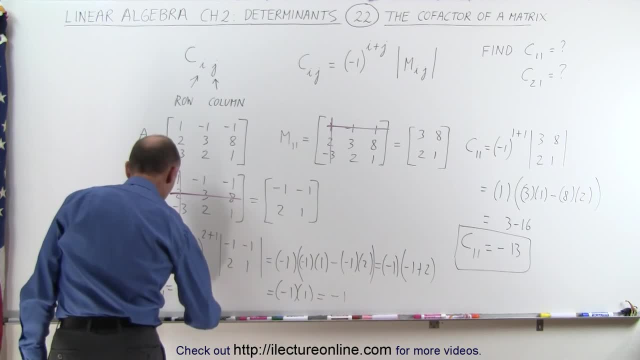 In other words, C21 equals, in this case, a minus 1.